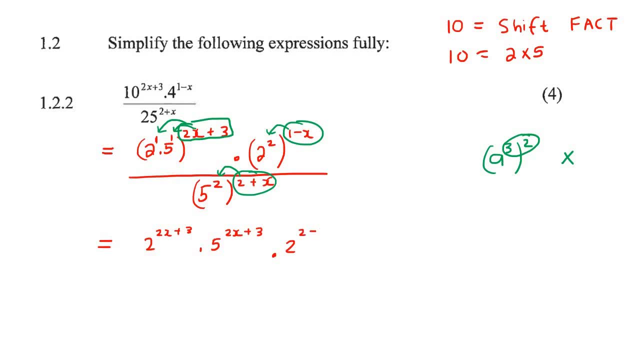 of 2 minus whoopsie, 2 minus 2x, 2x. And then, at the bottom, we're going to end up with 5 to the power of 2,, sorry, 4.. Come on, Kev, 4 plus 2x. Okay, now what we do is we look at the top. Okay, so just look at the top, Do you? 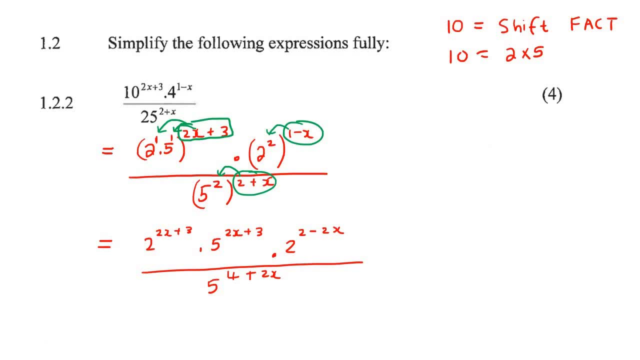 see anything, any terms that have the same base? Well, yes, these two over here. they are the same. So what would you do with this exponent rule over here? If you have a3 and then you have a2, how does the exponent rule work? Well, you keep it as a, so you don't change that. And then what? 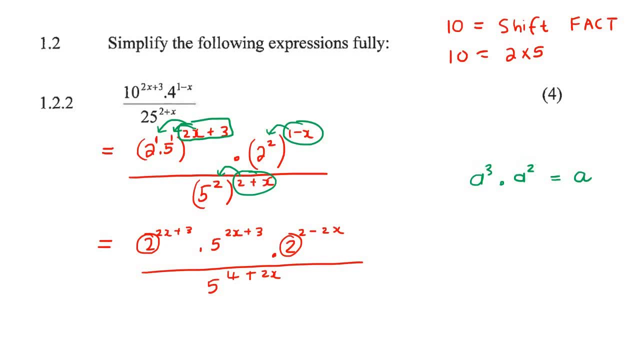 do you do with the 3 and the 2?? You add them together So that'll become 3 plus 2, and so this is going to be a to the power of 5.. So what we'll do, because what a lot of students want to. 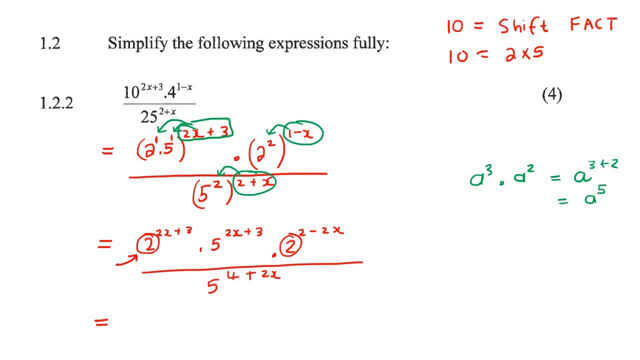 do is they want to take this 2 and this 2, and they want to turn it into a 4.. So they want to say 2 times 2 is 4, but that's not what we did here. We kept this number at the bottom as the. 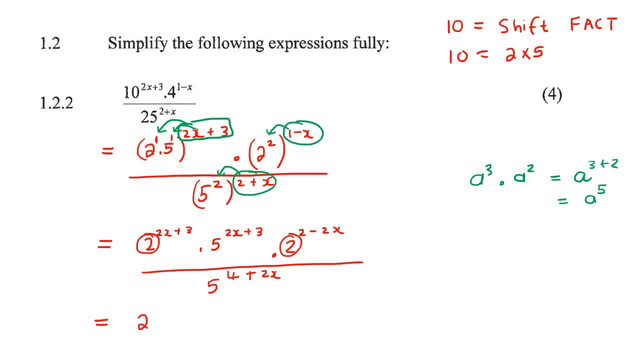 same. So you're going to say 2 times 2 is 4.. So you're going to say 2 times 2 is 4.. So you're going to say 2, and then you're going to add these exponents together, So that's going to be. 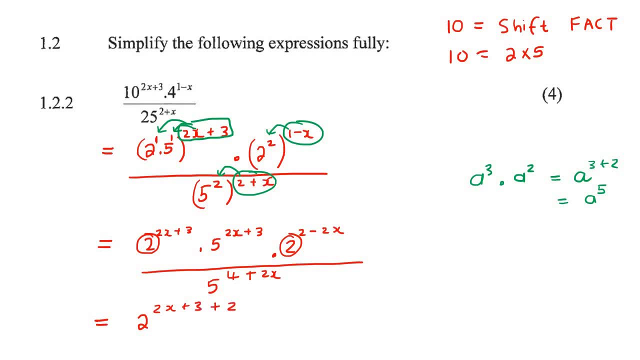 2x plus 3 plus 2 minus 2x, And then this one is going to be 5.. Well, I'm going to run out of space. Let me just move this up a bit. So it's going to be 2 to the power of 2x plus 3 plus 2. 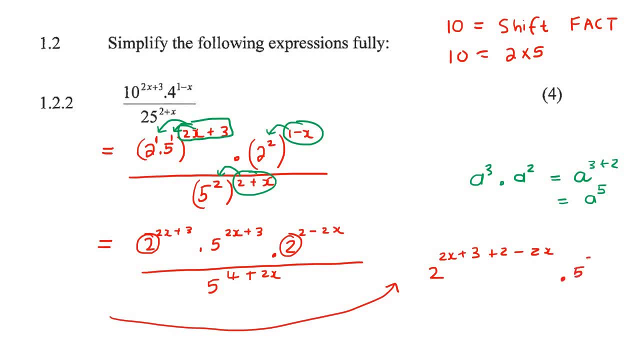 minus 2x, And then we'll be left with the 5, which is still there, Okay, And then at the bottom it's going to be 4 plus 2x. All right, I decided to move it over here, So now what I'm going to do. 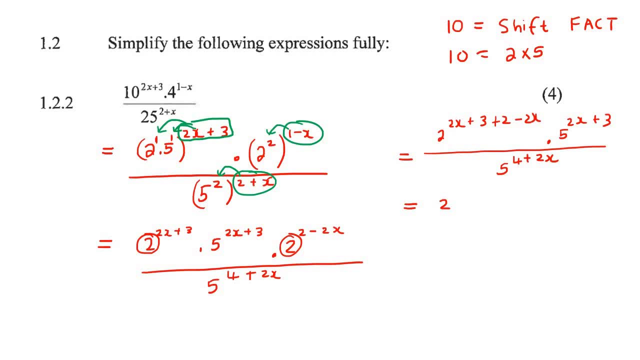 is, I'm just going to combine all of this So that's going to become 2 to the power of. oh, the 2x and the minus 2x they would cancel. So we just end up with 2 to the 5. And then we still. 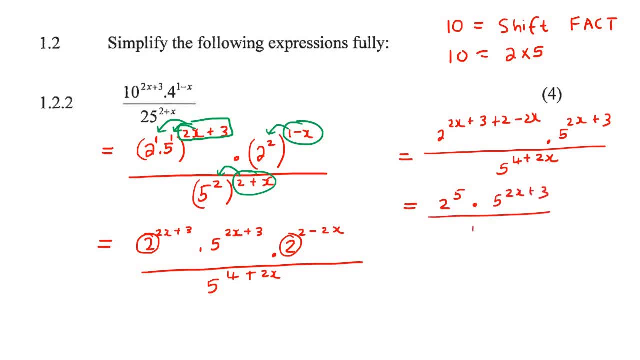 have the 5 to the 2x plus 3.. And then, at the bottom, we still have the 5 and then 4 plus 2x. Okay, So now what exponent rule? what would you do with an example like this? 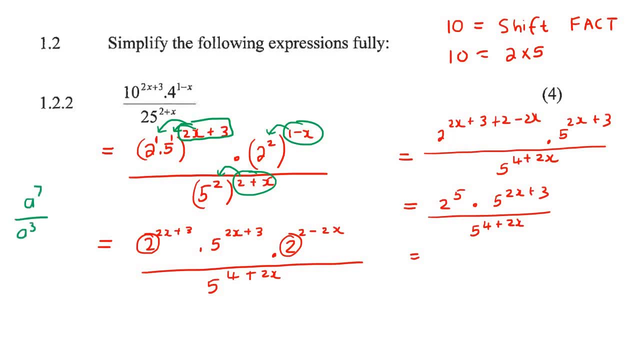 You have, for example, a7 over a3. Then what do you do with your exponents? You minus them. So 7 minus 3 is 4.. But you don't change the a. What a lot of students try to do here is they want to. 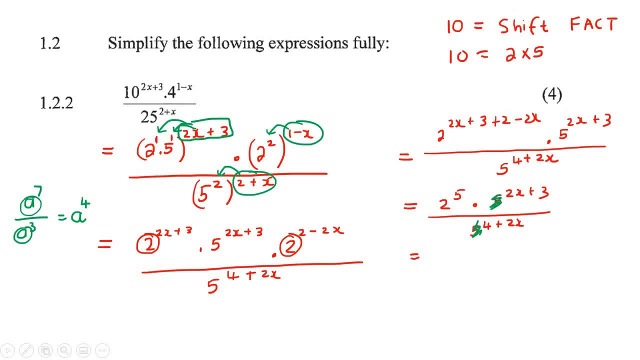 cancel out the fives, But that's not correct. If it was a 5 by itself, then of course you could cancel them, But because they are exponents, we have to stick to exponent rules, Okay, So what we're going to have now is we're going to keep that as 2 to the 5. And then we're going to say: 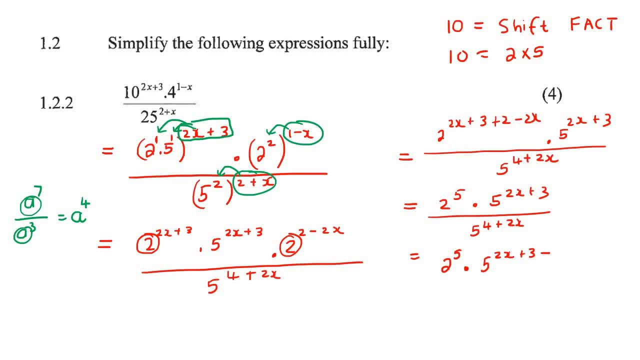 5 to the 2x plus 3 minus. then we're going to say, in brackets, 4 plus 2x. You see what I did. I took these top exponents minus the bottom exponents, And so that's going to be 2 to the 5.. 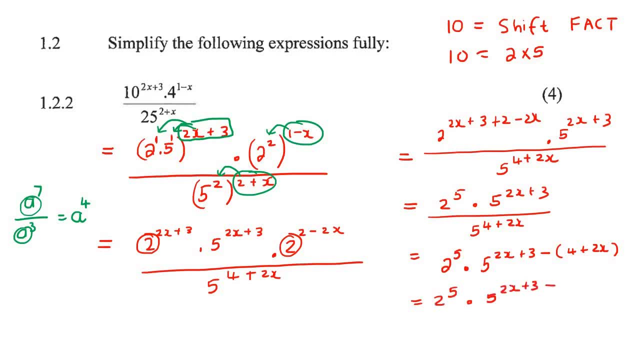 And then this is going to be 5 to the 2x plus 3 minus 4 minus 2x, And so that'll be 2 to the 5. And then these two x's are going to cancel, And then you're going to have 3 minus 4, which is: 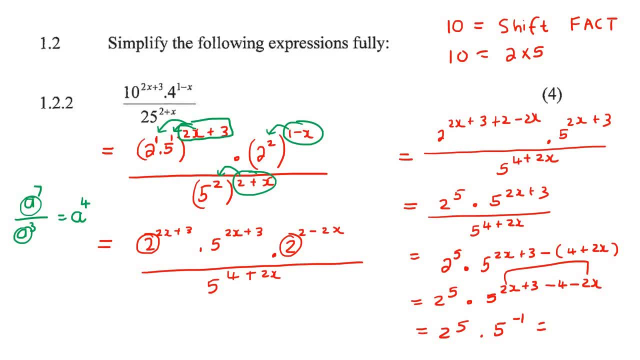 minus 1.. And so what we then do is we're going to cancel out the fives, And then we're going to, because we don't want to have negative exponents. So what we'll do is we'll put that back down at the 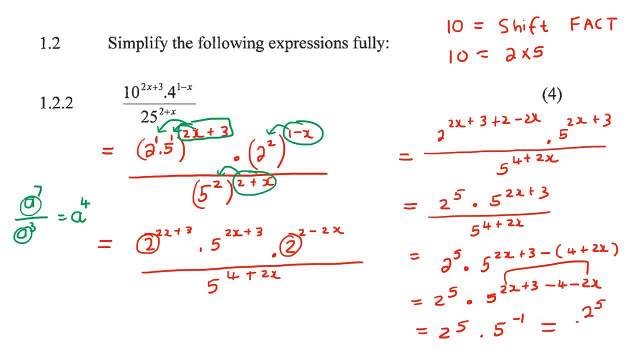 bottom. So we'll say 2 to the 5 and then over 5 to the 1. And then we could work that out. So 2 to the 5 is 32.. So sorry, I'm going to write the final answer here. The final answer then would: